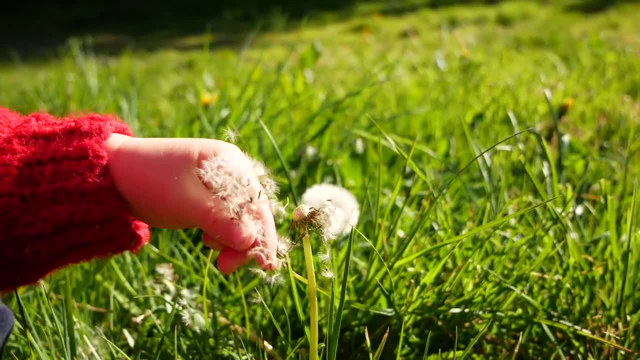 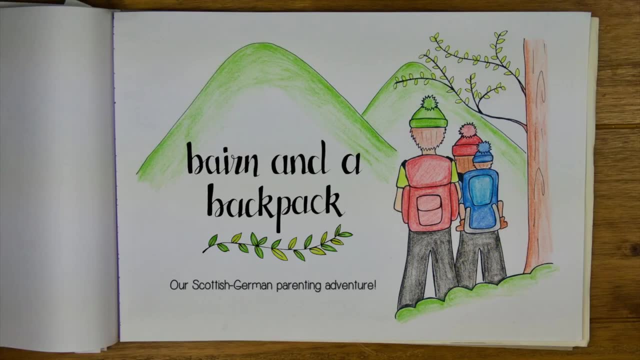 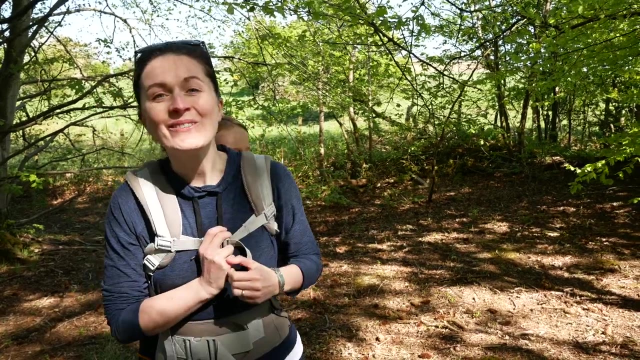 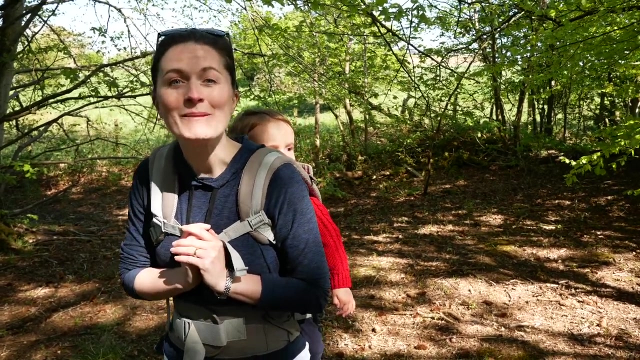 Hi guys, I'm Cara. I'm mum to this little 21 month old here called Ben, and I post videos about being a toddler parent twice a week, so make sure you're subscribed, if you've not already. In today's video, we are out and about on our daily walk. Luckily, we live very close to a forest and that's where 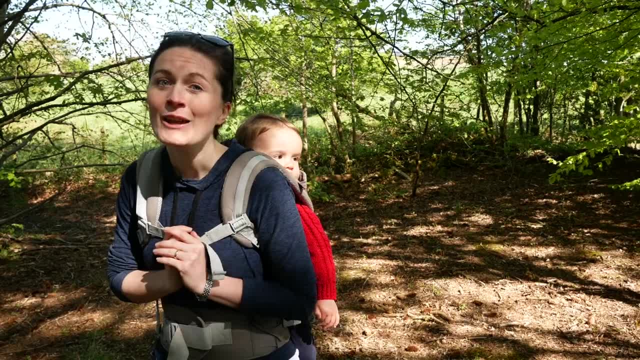 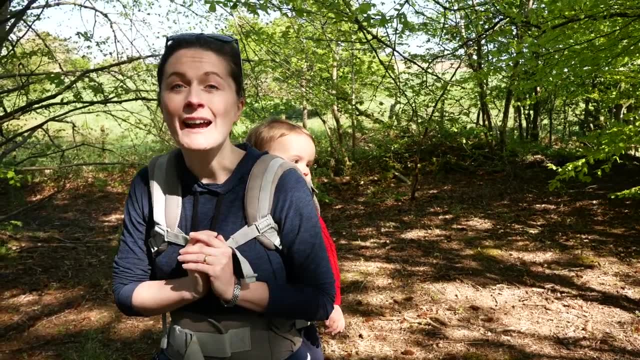 we've been doing lots of our daily exercise. that's really beautiful. So we're going to be showing you some of the activities we do while we're out on our daily walk, and we're also going to be taking some things back to do some craft activities at home, which we'll be showing you. 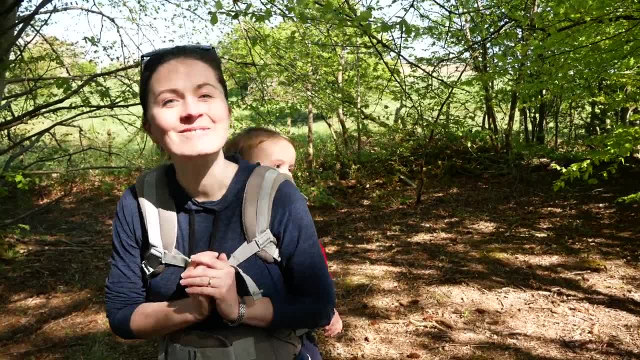 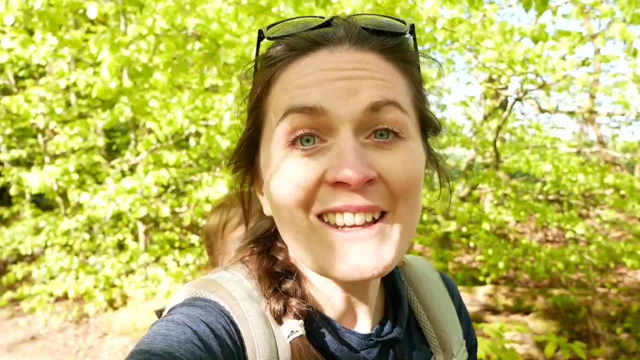 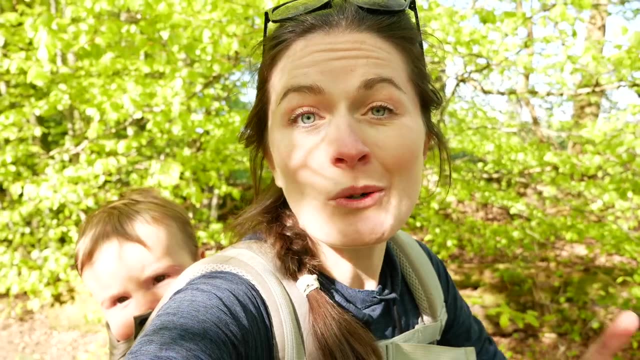 later on in this video as well. so make sure you stick around. So let's go. So the beauty of all of the activities that I'm going to do today with Ben is that you can totally adapt them to whatever outdoor space you have. We don't have a garden, so the only outdoor time that 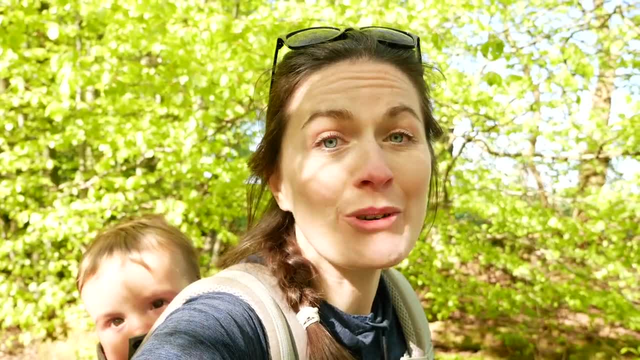 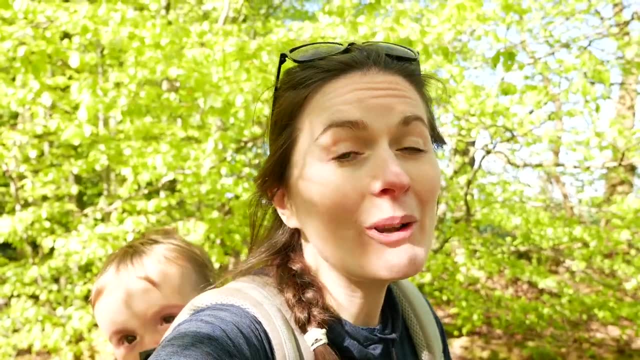 we have at the moment is during our daily exercise, but we are lucky enough to live really close to the forest. But these activities can be recreated in your garden, in a local park, even out and about in your neighbourhood, and just do what works for you. 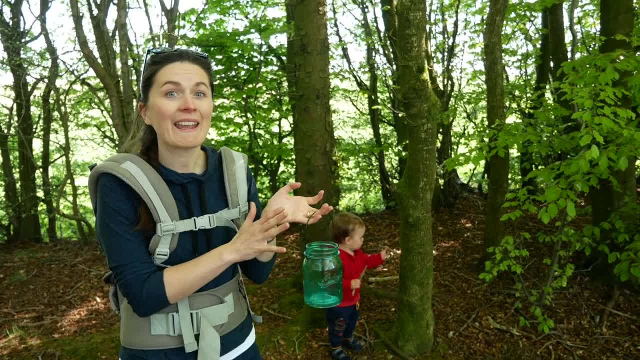 One of the things I do is bring along a little glass jar with a handle and make it like a treasure jar so Ben can fill it with all of the kinds of things he finds in the garden. So I'm going to show you some of the things that I find interesting and then we can use them for craft. 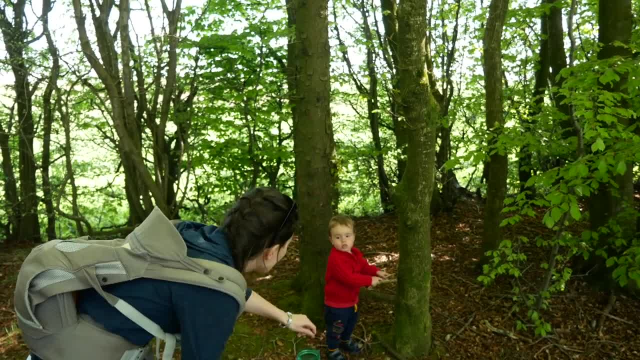 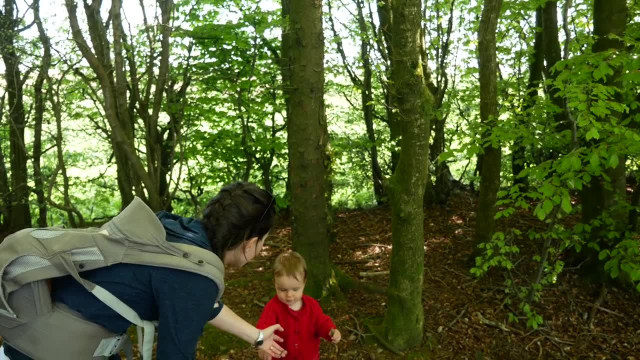 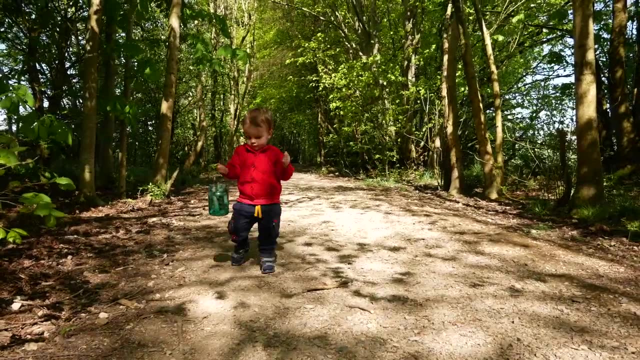 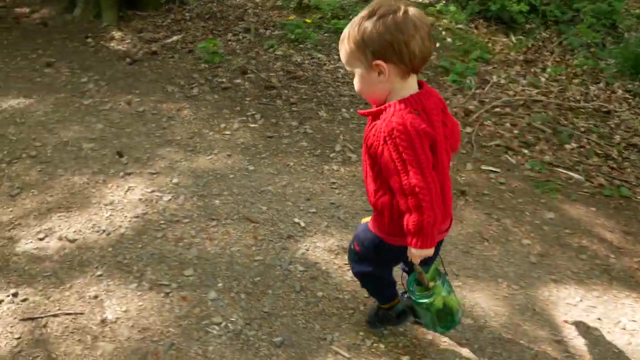 projects when we get back home. So, Ben, where's your jar? Do you want to put your stick on the side? So Ben is really loving his little jar. If you don't have a jar like this at home, you could also use a basket or a bag, or even a little bucket. 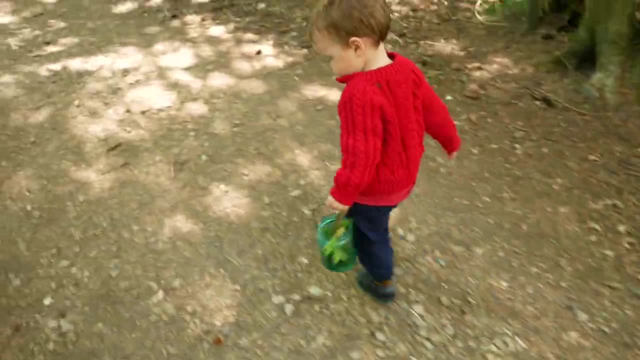 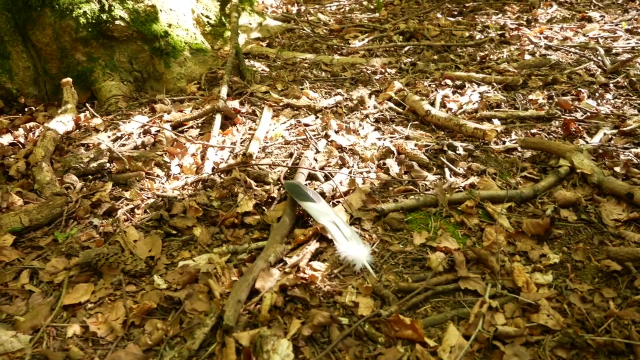 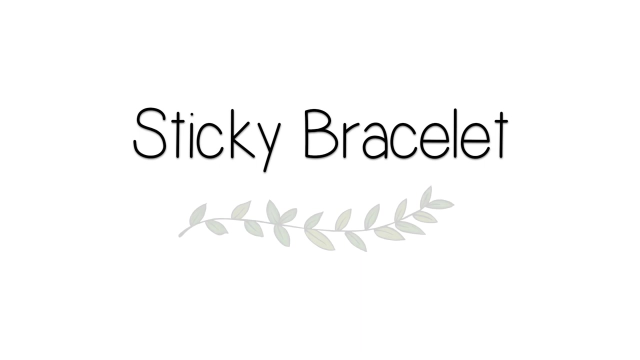 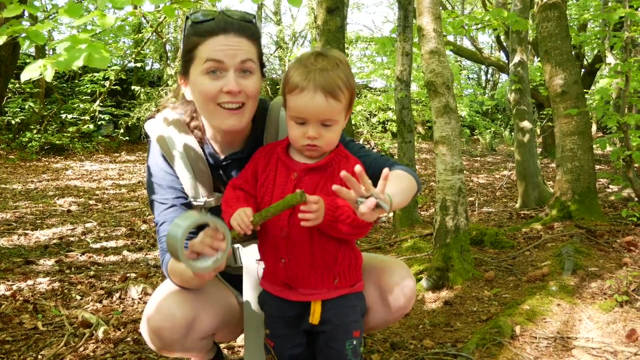 And he's loving collecting all of his little treasures to take home with him. Ben, what do you have in your jar? Sticks, Sticks. What else? Leafs, Leafs, Feta, Feta. So for the next activity, all you need is some tape. I'm going to use duct tape, but you could 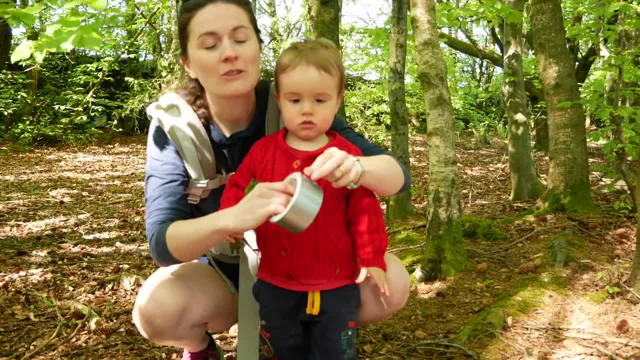 use masking tape or sellotape, whatever you have in the house. So you just need to take a little piece of tape and put it in your jar, and then you can put it in your jar, and then you can take a little piece of tape and put it in your jar, and then you can put it in your jar, and then you can. 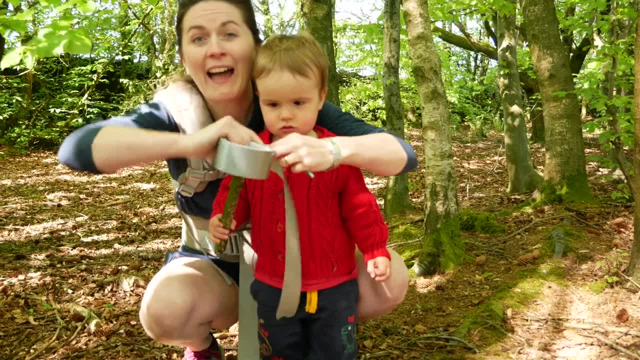 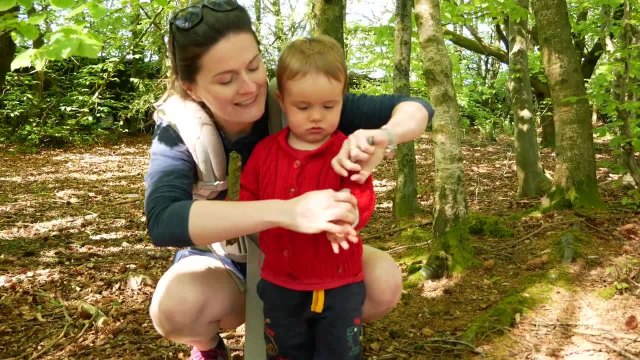 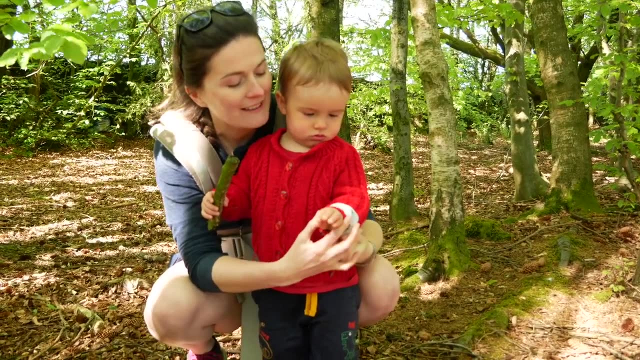 take another piece, rip it off and put it around your toddler's arm so that they have a sticky bracelet. Oh look, you have a sticky arm. Wow, We're going to add whatever you want to stick to it as a special treasure. So look, if we want to stick a beechnut to it. 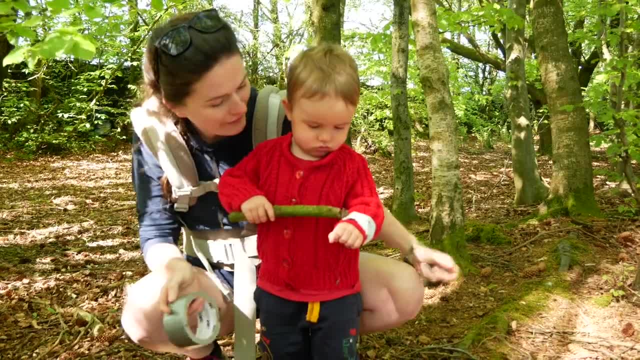 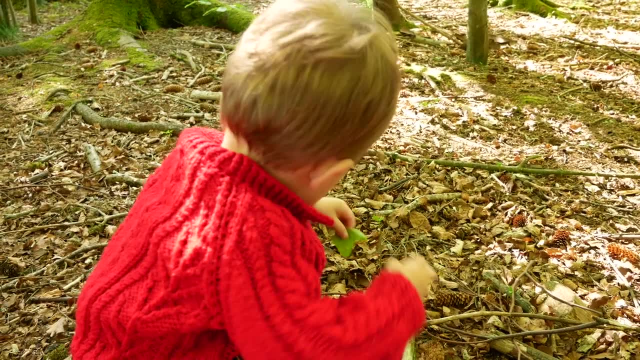 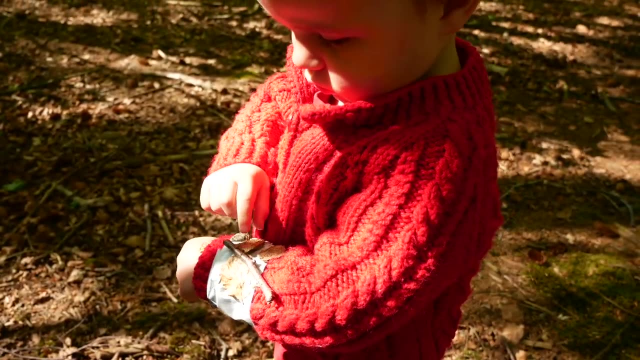 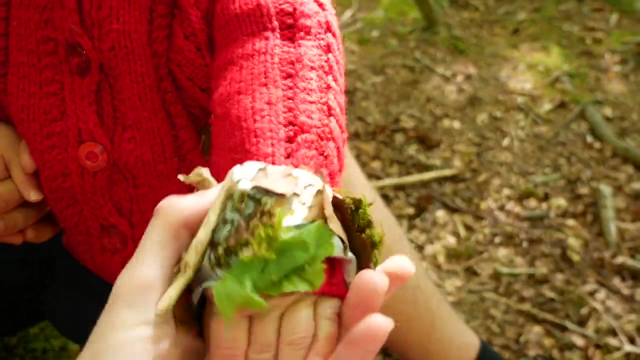 we just go pop and it's stuck. Or you could stick a leaf, And here is Ben's beautiful woodland bracelet. I'm going to stick a big and nice little housie bracelet into the jar and then I just want to put some of the stuff in there. 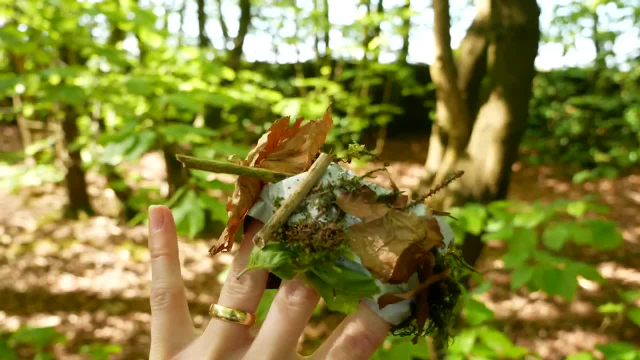 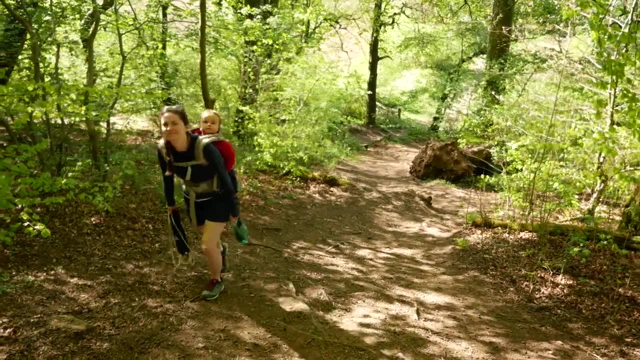 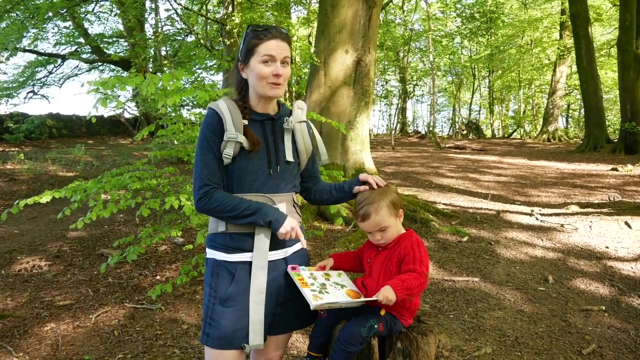 And here is Ben's beautiful woodland bracelet. I'm just going to put some flowers in here and then I'm going to wrap it around the tree. I'm going to stick a half-moon-tall satin bracelet in my jar. another thing that we really love to do is have a picture scavenger hunt. so we have this nature. 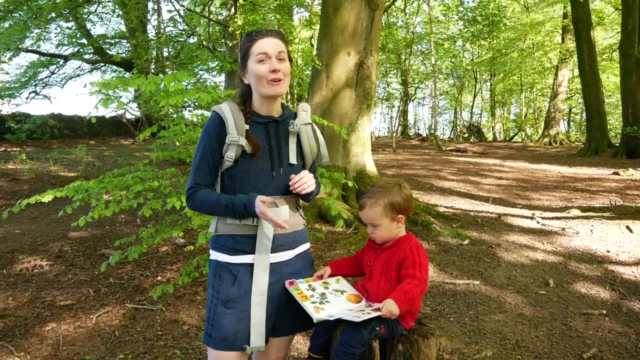 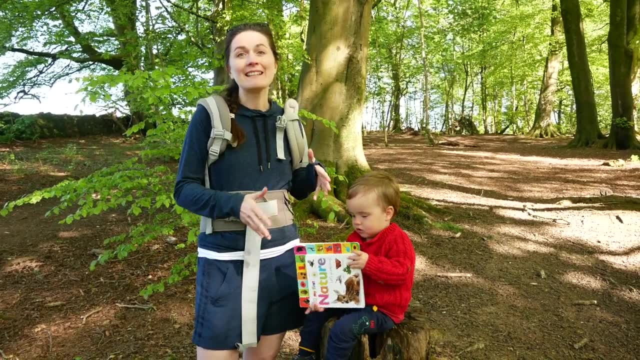 book from DK. I really, really rate their picture books. we have quite a few of them and they're really great for language development and for lots of different types of activities. so we'll show Ben one of the pictures and then together we'll go and look for that thing. if you don't. 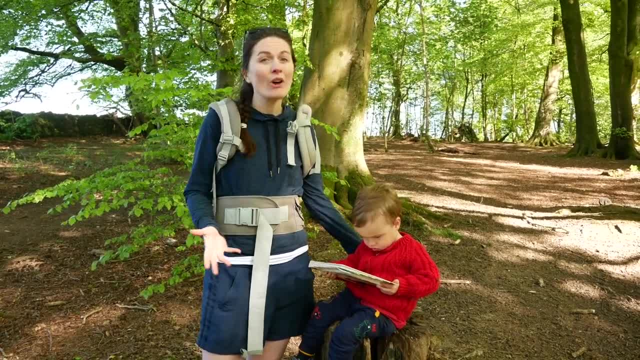 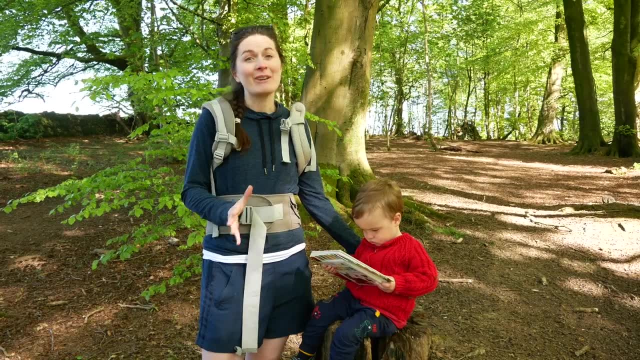 have a nature book like this. you could also just use pictures that you've drawn or pictures from the internet and create your own little mini flashcards or scavenger hunt sheet, and it's really great fun and we can all do it together. here we've got some leaves. do you think you could? 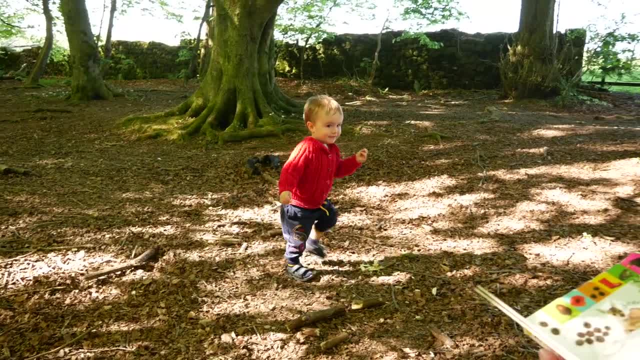 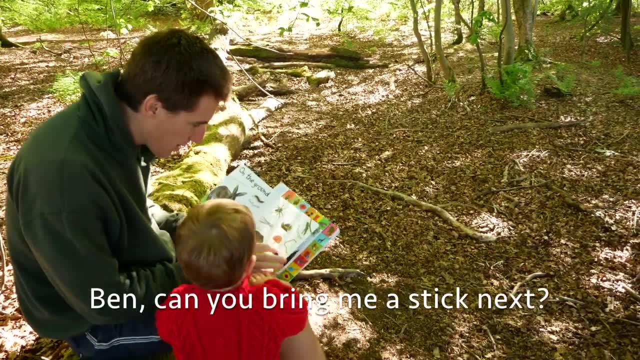 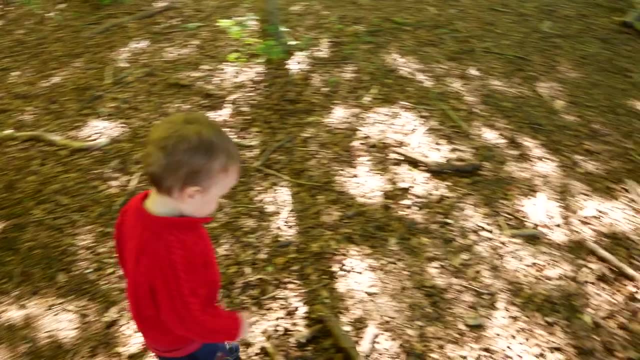 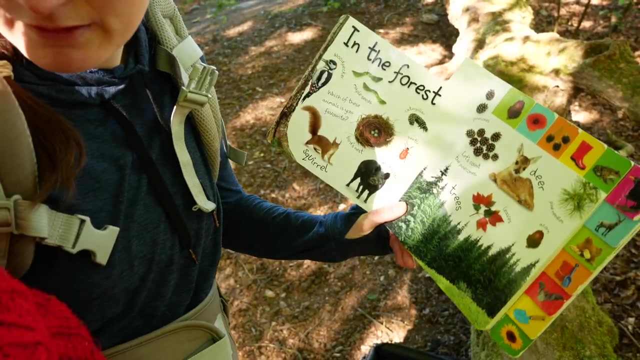 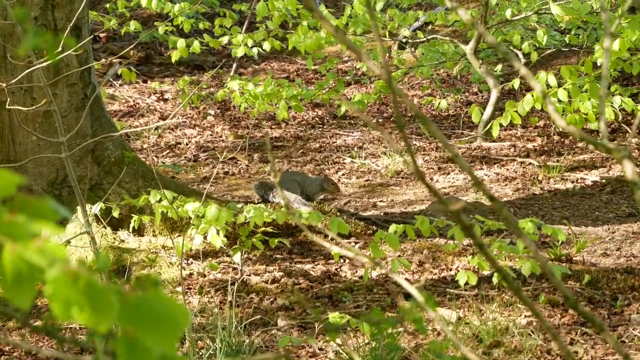 bring me a leaf. thank you, and can you bring me a stick next time? can you bring me a stick? thank you, a stick. shall we look for a squirrel? as far as the scavenger hunt is concerned, it doesn't have to be squirrels and mice, like what. 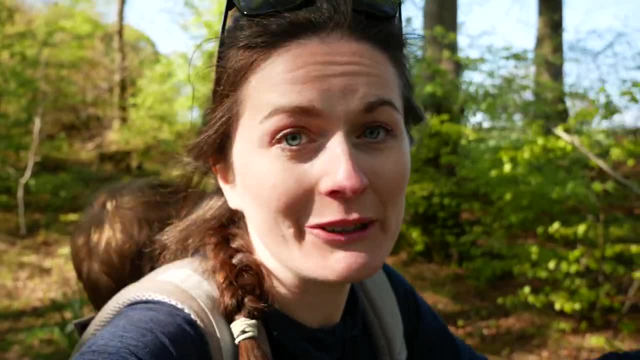 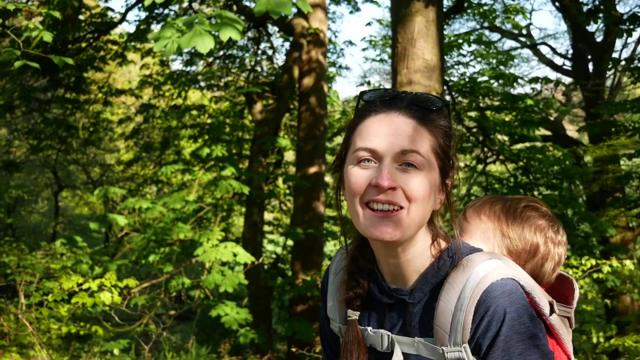 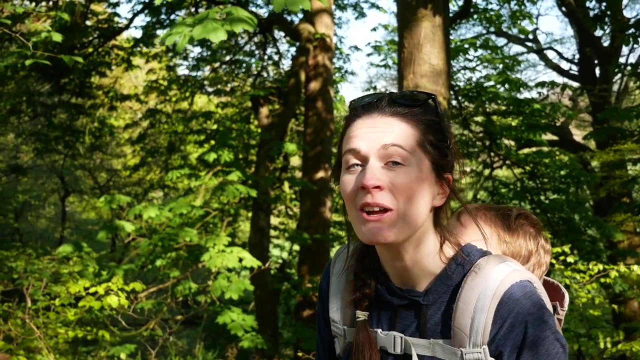 we see here in the woods. it could be a certain color of car or a traffic cone. and my final game is a very simple version of I spy. obviously Ben is too small to know letters yet. he's just starting to recognize colors, so right now it's just a. 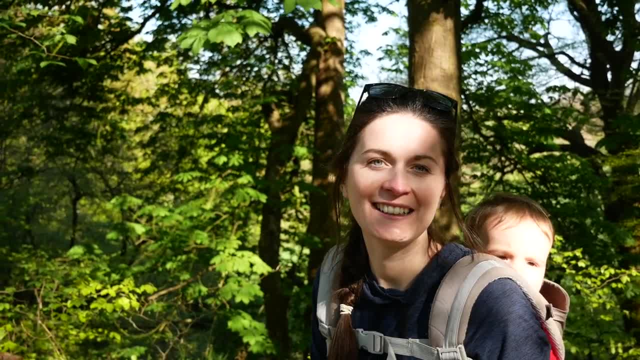 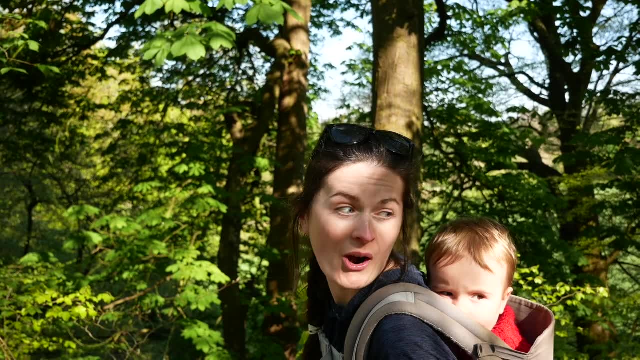 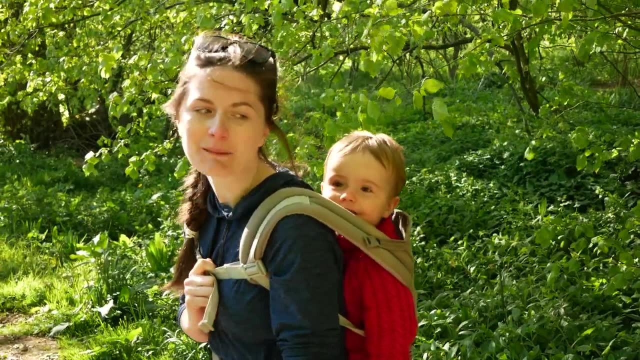 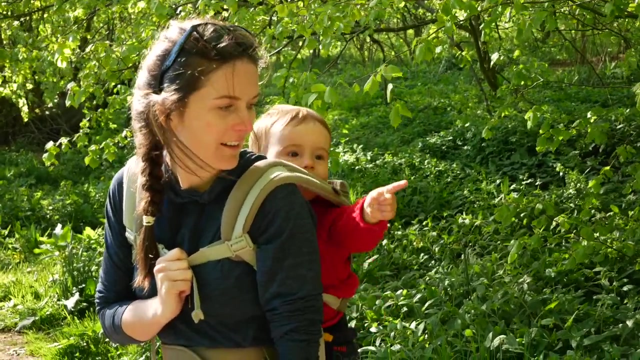 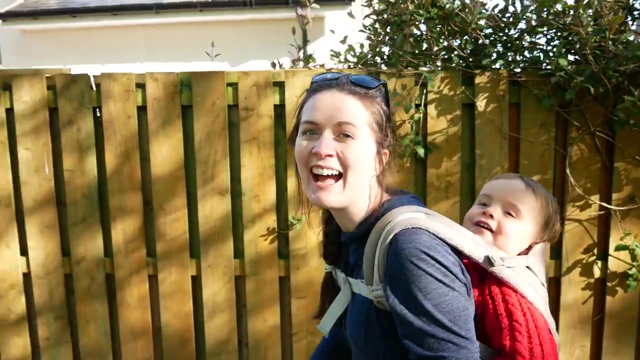 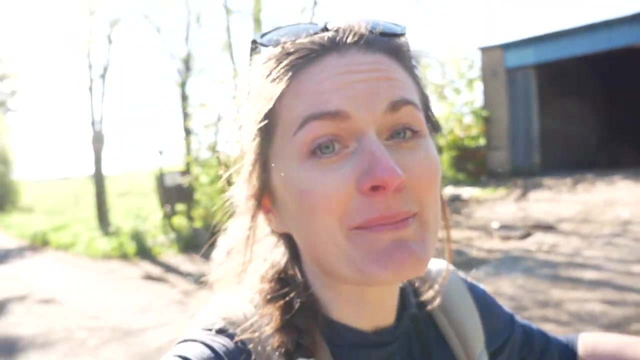 a game of recognition while he's such a young toddler. Ben, do you hear the woodpecker? I spy with my little eye- a grass, can you see some too? where I spy with my little eye: a field. can you see one too? the I spy game is a favorite for us when we actually need to get somewhere. so now Ben's in. 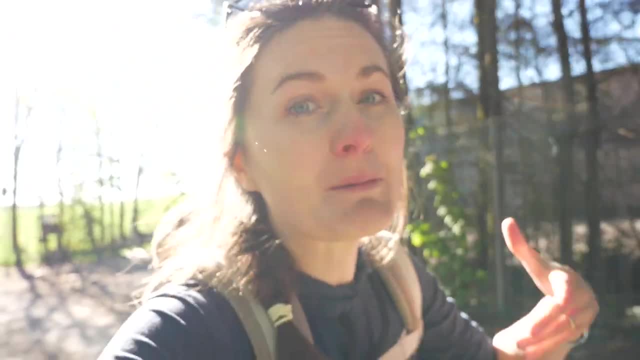 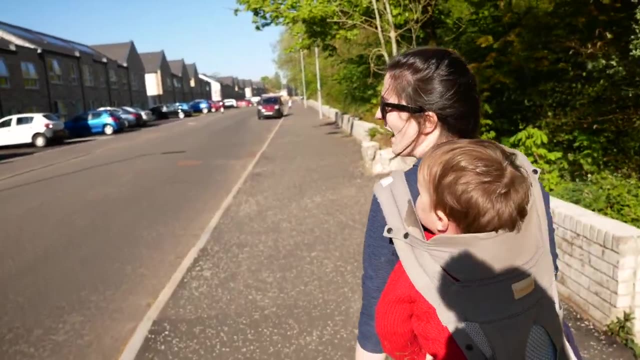 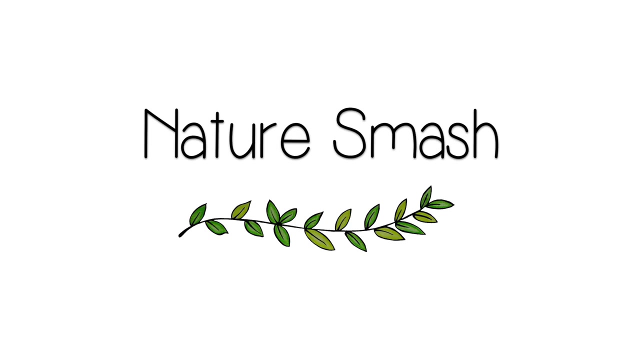 the backpack because we're going to get home and get dinner on um. so it keeps him really occupied while we're walking through the town. and well, he's just sitting. still, I spy with my little eye. a car, do you see one too? yeah, car, om. so it's now the next day and the weather today is not nearly as good as it was. 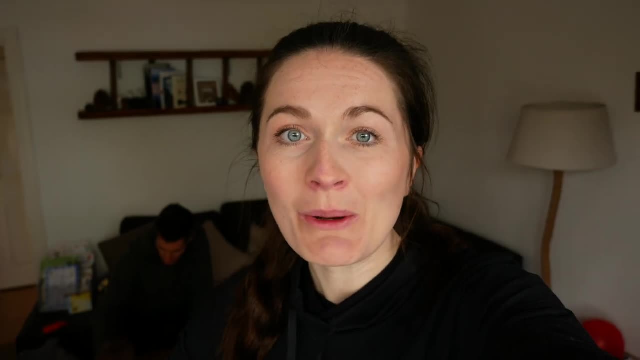 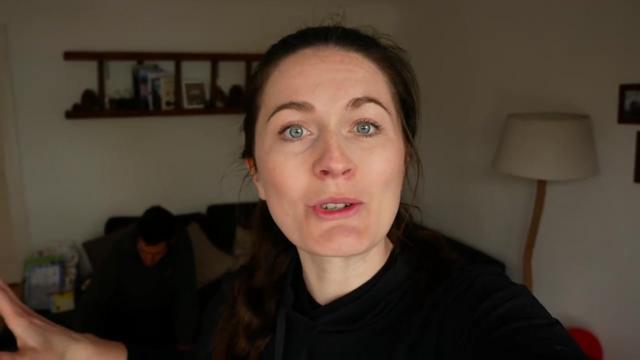 yesterday, so I'm really glad that we were out and made the most of it. today we're going to be using some of the things that we collected yesterday for some crafts and activities, and the first activity is just set up over here, so I'm going to show you what that is. 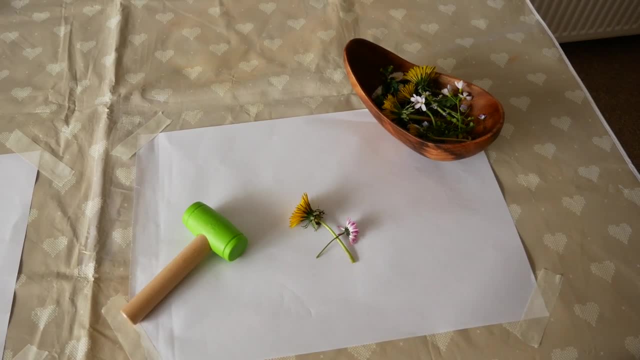 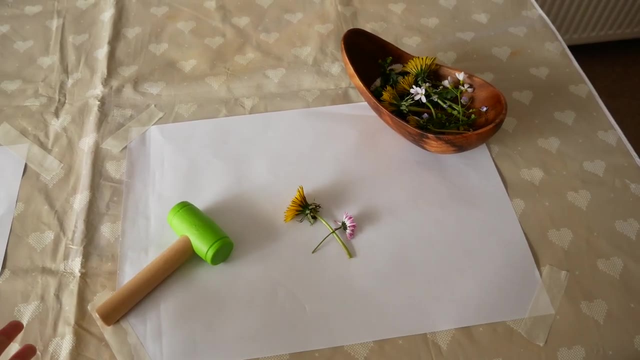 Nature Smash activity. so Ben has got a little wooden Hammer here- that's from one of his hammering toys- and I've got a little bowl of flowers that other people would consider to be weeds. The idea is that Ben's going to smash them. the colours will come off and we'll make some really nice pictures. 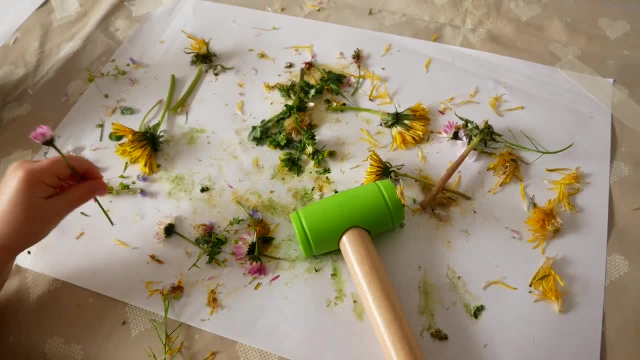 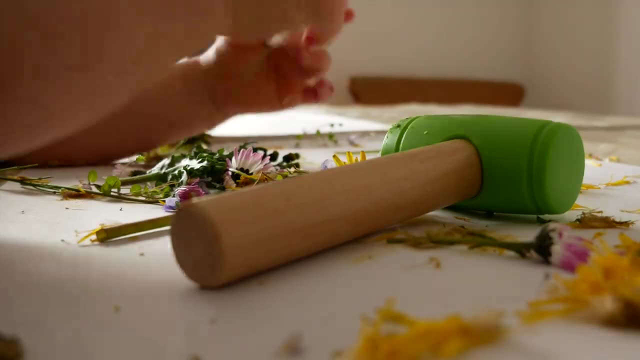 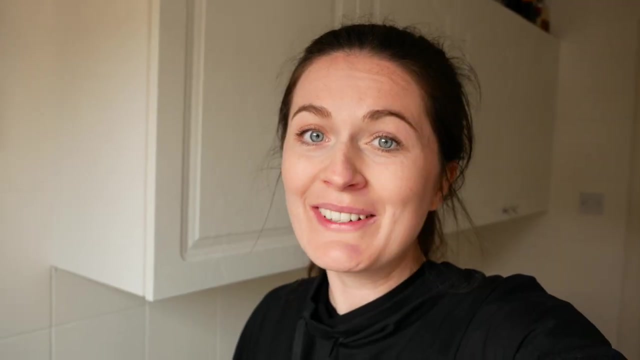 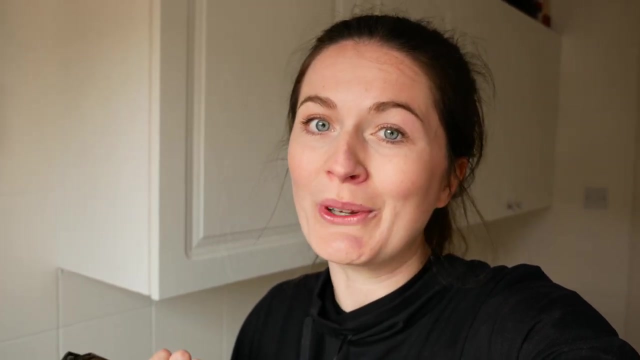 So, as you can see, this doesn't make the most beautiful picture in the world, but it is a process that Ben is really enjoying. My next activity is honestly the easiest activity to set up. I actually did a version of this activity in my language activities video, which I uploaded last week, so I'll link that below in case you want to check that out as well. 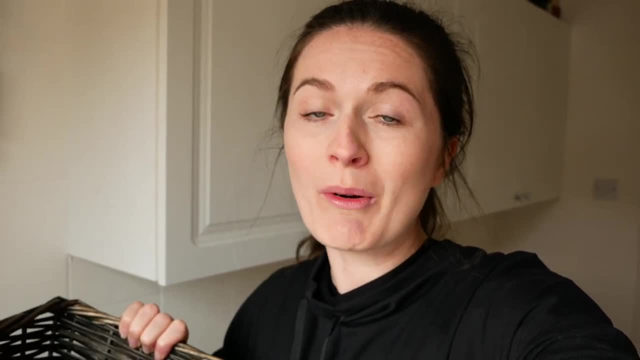 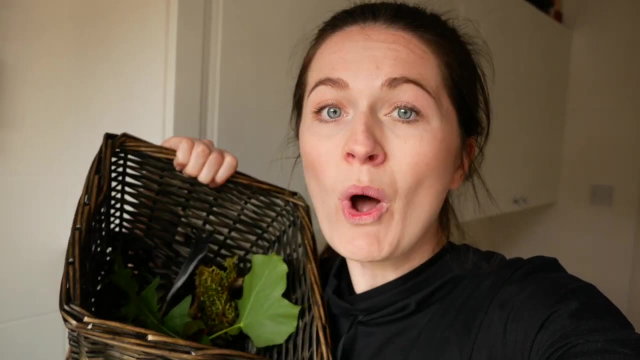 But I've got a nature talking basket, So all I've done is take some of the things that Ben collected in his little glass jar yesterday, some of the things that I collected in the cloth bag, and put them in a basket. All we're going to do is have a chat about them. 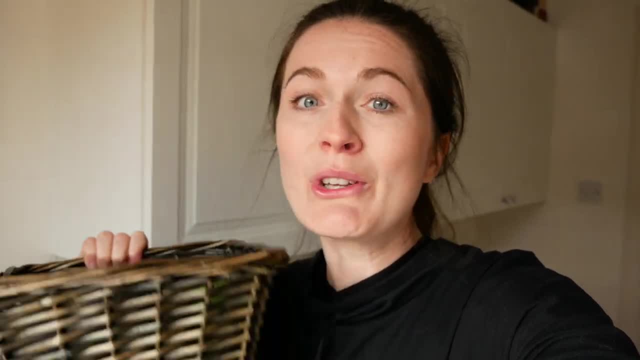 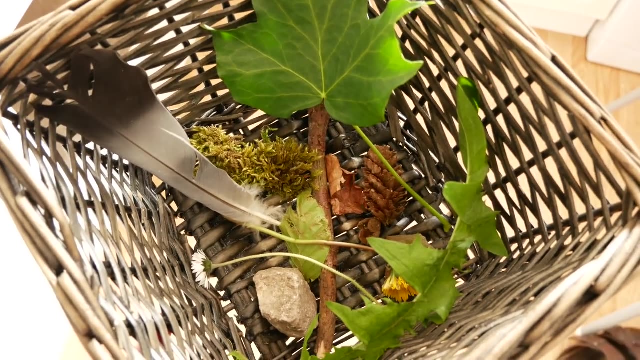 Some of them. I know Ben already knows the words for some of them he doesn't, and we're just going to explore them together. So, as you can see, it's just filled with some super simple things: A feather, an ivy leaf, a dandelion leaf, a daisy, some moss. 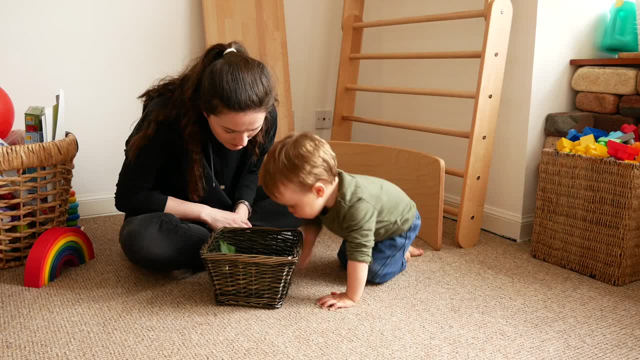 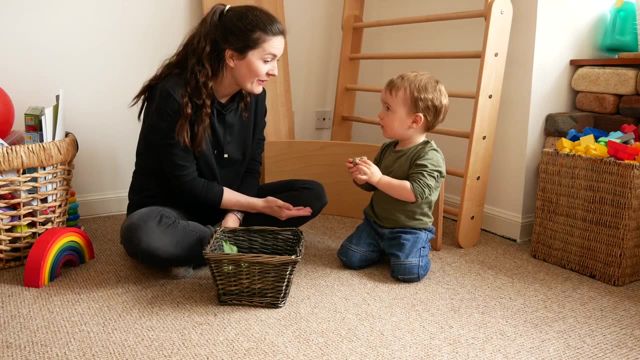 What's in here? A stone, A stone, Plop, Plop. Yeah, we plop it in the water, don't we when we're out for a walk. Can we take that with us on a walk today, Yeah, 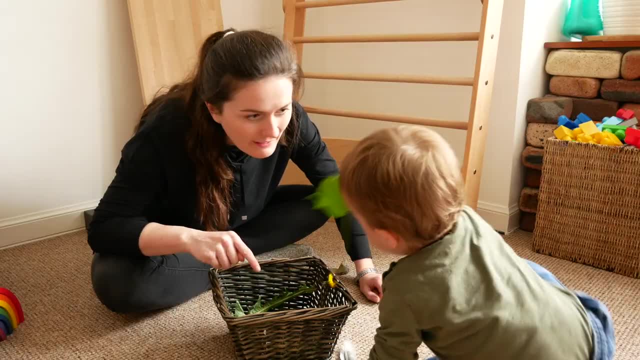 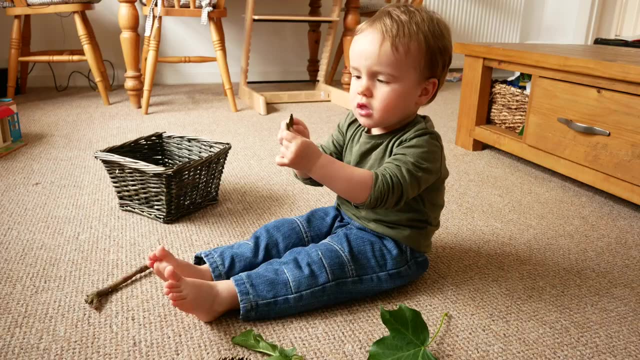 Yeah, And plop it in the water, Yeah, OK, And what's that? An ivy, Ivy Feather, A feather That's bark Dog. A dog barks, yes, but a tree also has bark Cone. 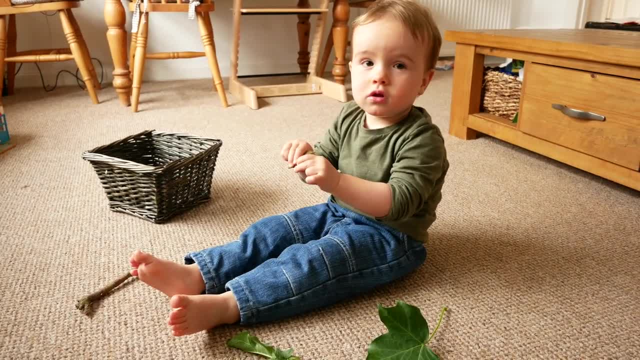 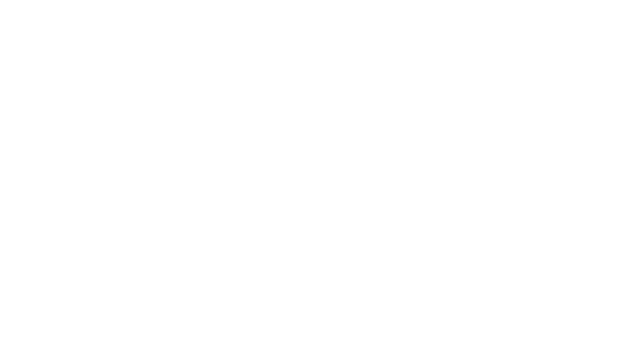 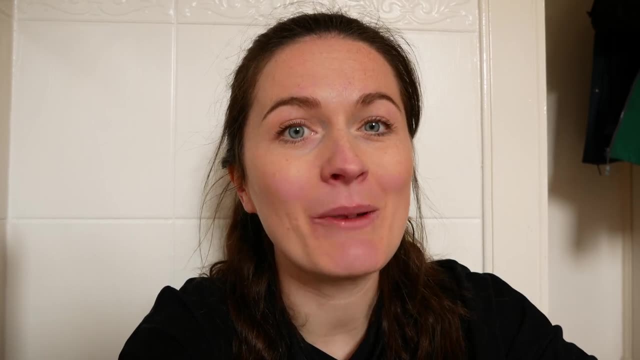 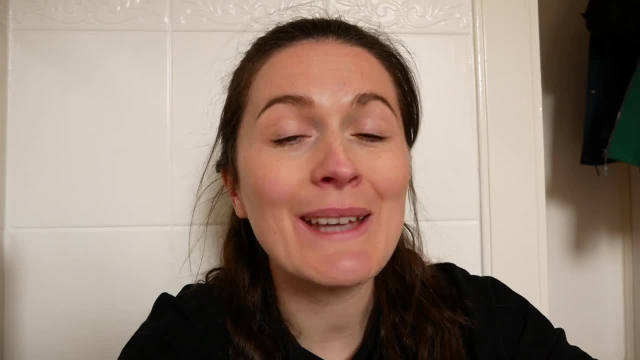 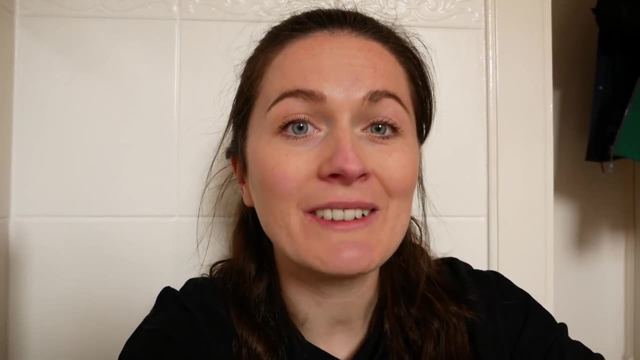 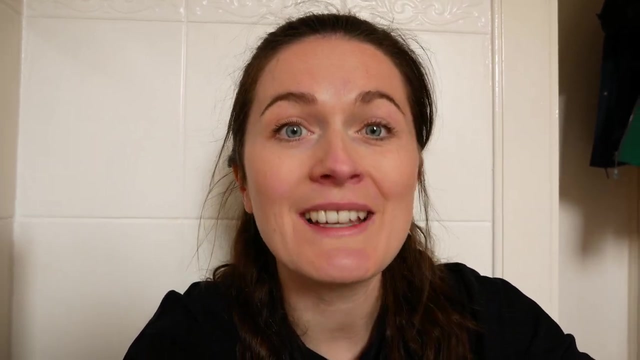 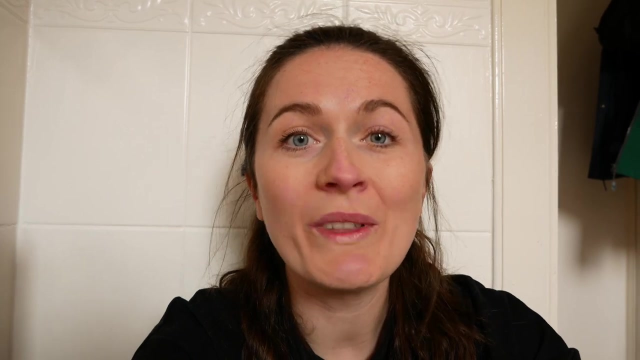 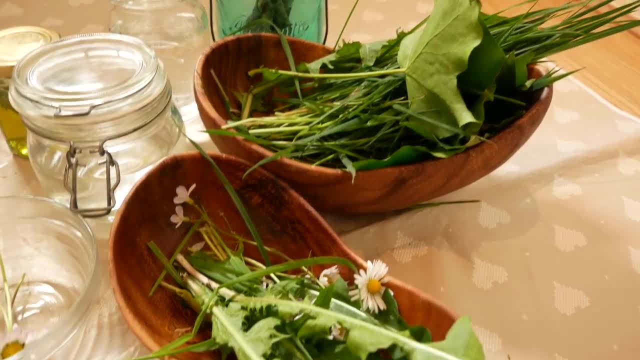 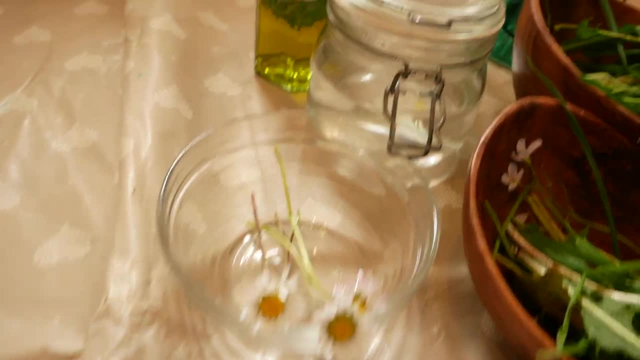 i just have two bowls filled with some of the things that we collected- some grass, some flowers- and i have lots of different bowls set out, so a little egg cup, a glass bowl here with some daisies in it and some jars filled with water. this one here is filled with, uh, water that i've decided. 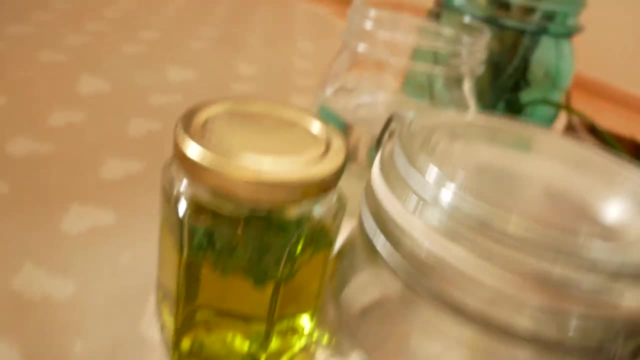 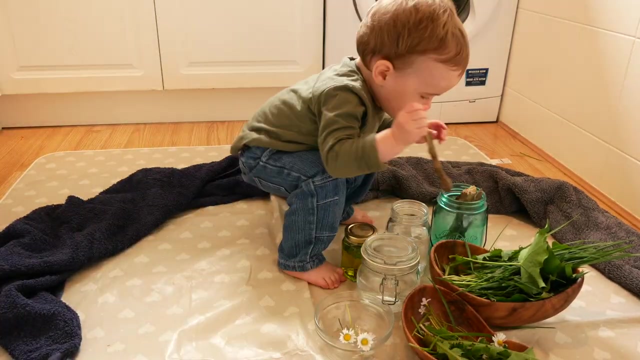 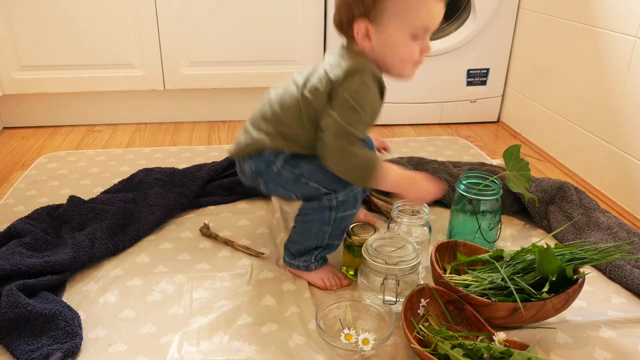 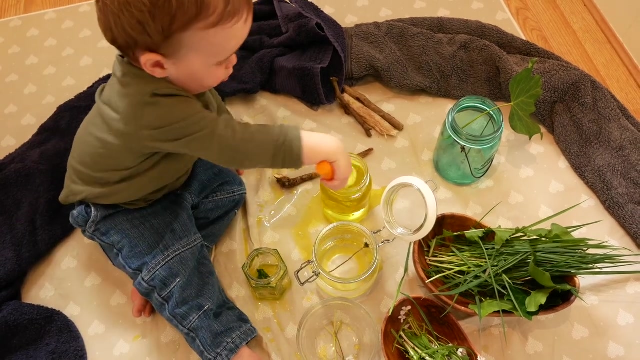 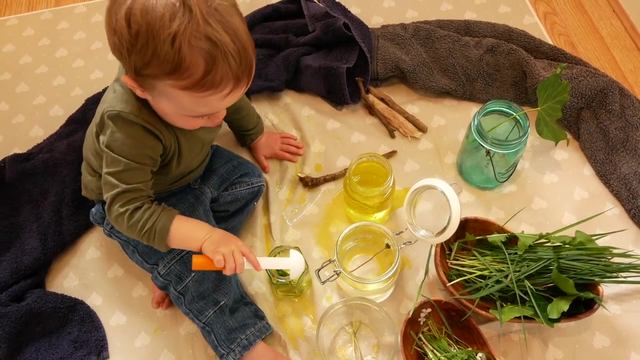 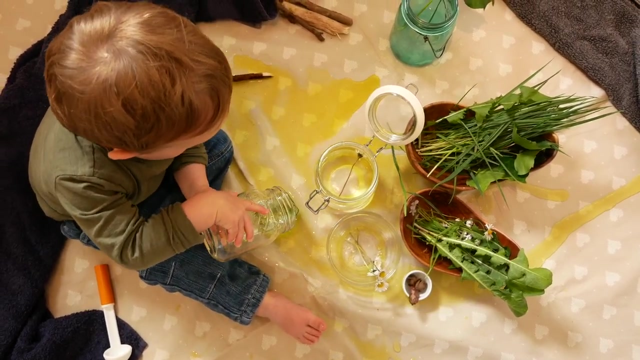 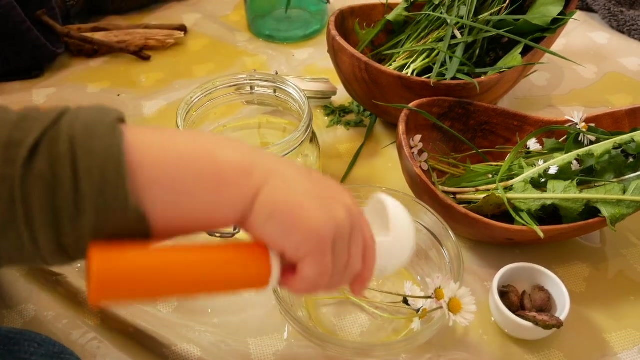 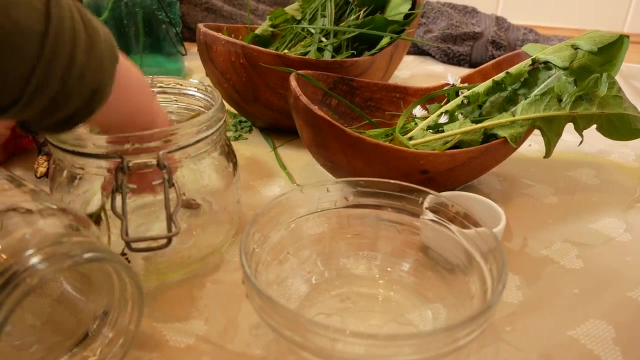 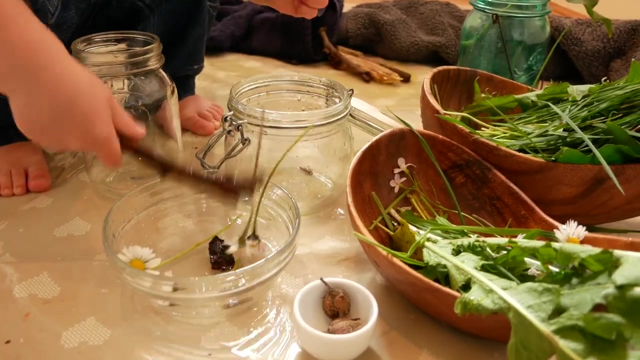 some green food coloring to and some of the kind of shrumpled up leaves that we collected yesterday. and then i also have some of his sticks that he collected in his jar, just so that you can use them as spins. so ben has been exploring this now for such a long time. it's so good for so many skills. 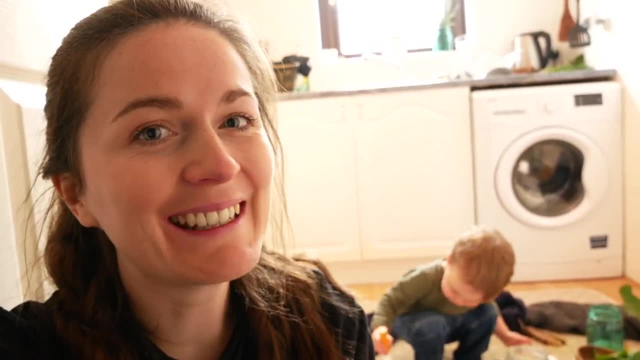 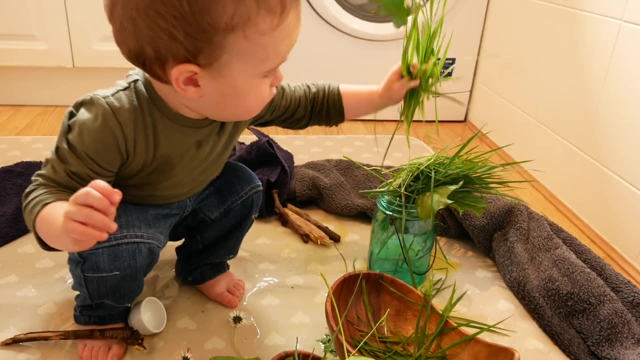 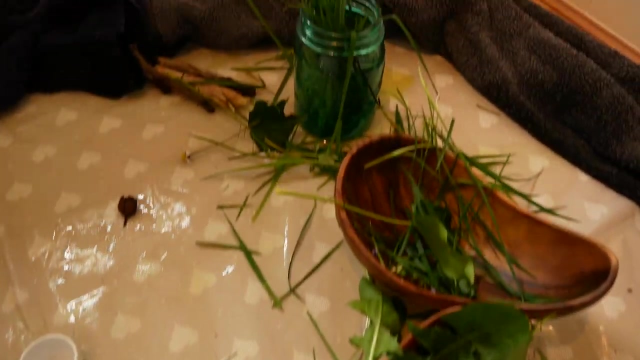 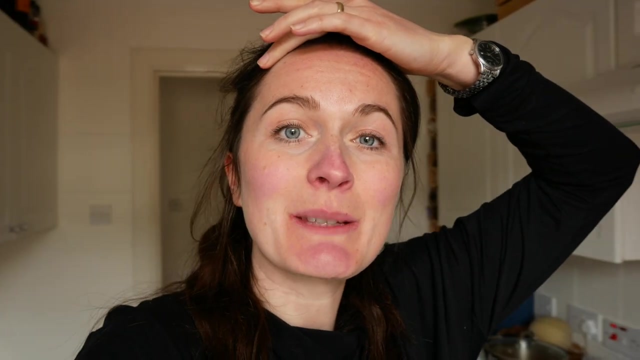 he's pouring lots, transferring things from one container into another, so it's an activity that he loves and that i really love for his development as well, and the aftermath looks a little bit like this, which i don't think is too bad. today is fast becoming a very exhausting parenting day. ben has been up since half. 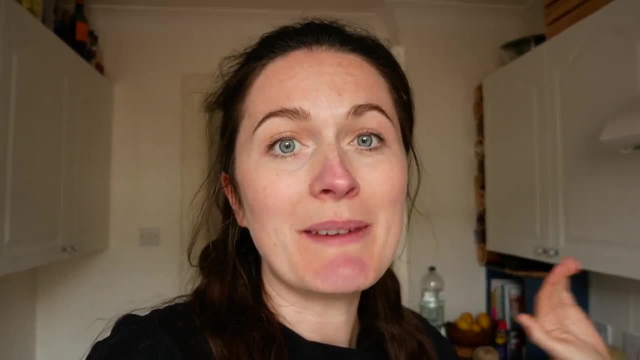 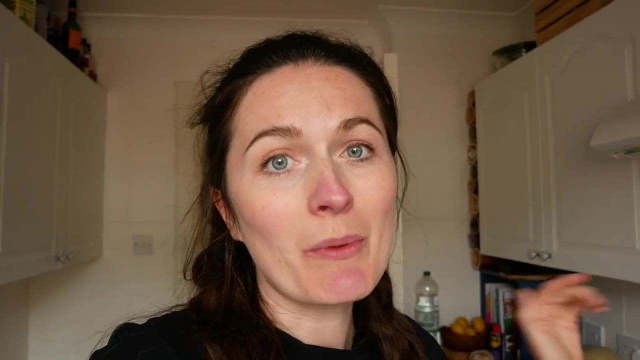 past five this morning. he's just refused any form of lunchtime nap, so he's going to be super exhausted and cranky and i'm not really sure how any more organized activities are going to go for today. but we will give our last activity a try in a wee minute. right now we need coffee. 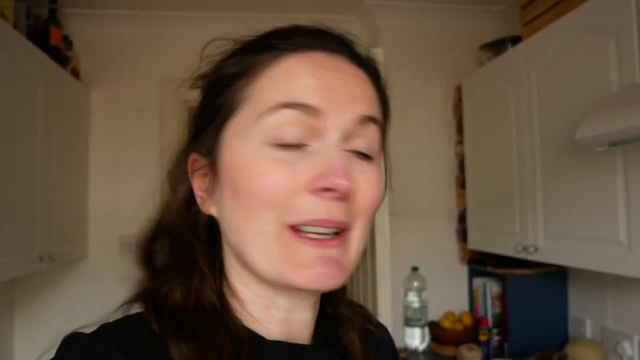 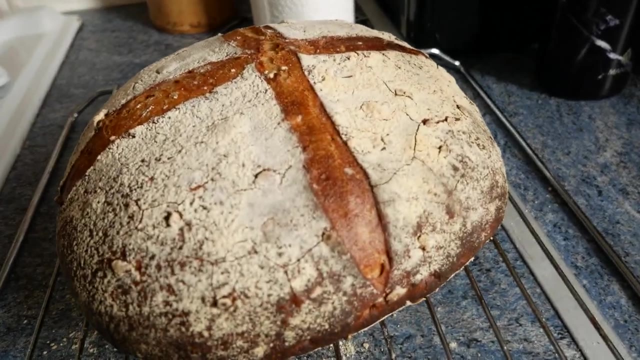 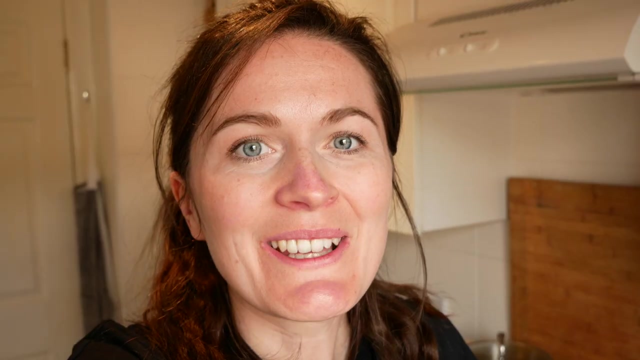 um, thomas has been really busy making this amazing looking sourdough bread, so we're really looking forward to tucking into that at some point as well. so the next activity is not for the faint-hearted. it involves paint and quite a lot of mess, but it. 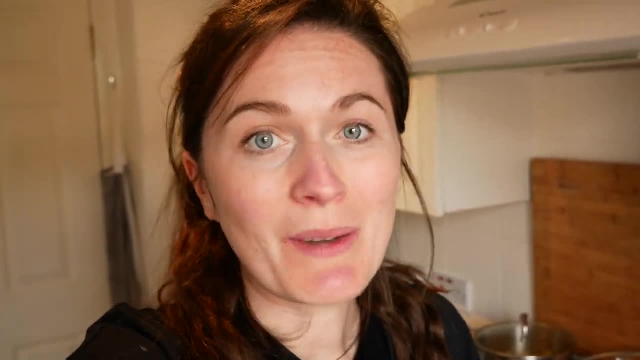 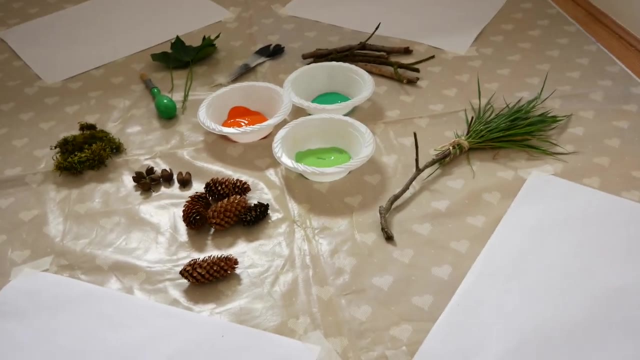 is something that ben usually really enjoys, so it's a nature printing activity. essentially, all i've done is set out some paint and some of the things that we gathered on our walk yesterday. so here's what i've set out for our nature printing. i've put my trusty tablecloth back. 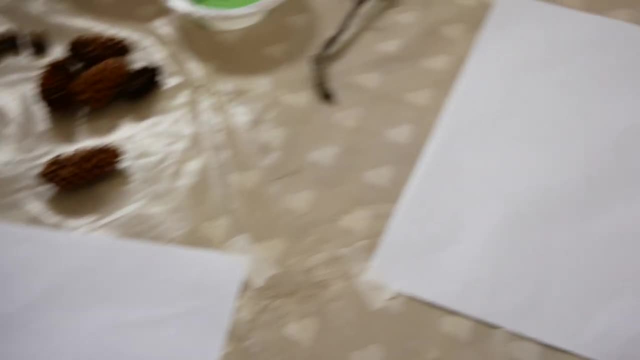 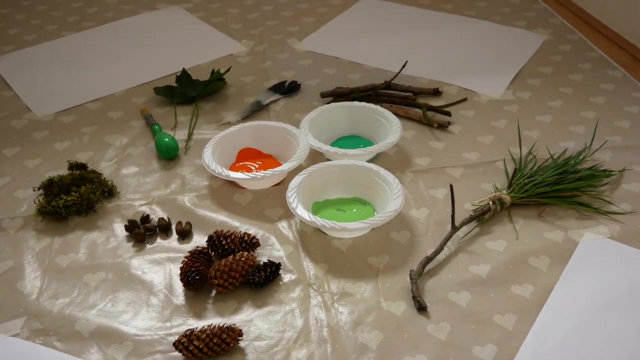 onto my kitchen floor and i have taped some paper to the cloth using some masking tape. i generally find that this works really well, because toddlers find it difficult to hold the paper and paint at the same time. then you'll see, i've put a range of the things that we collected yesterday and 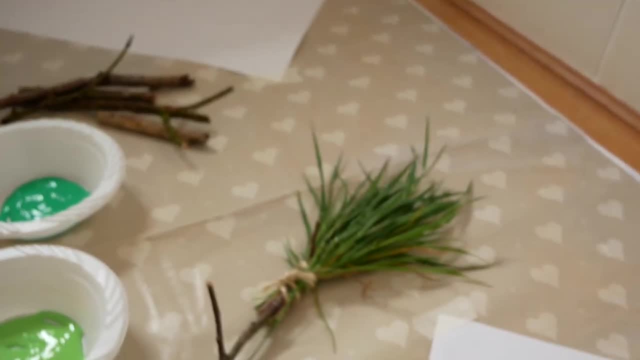 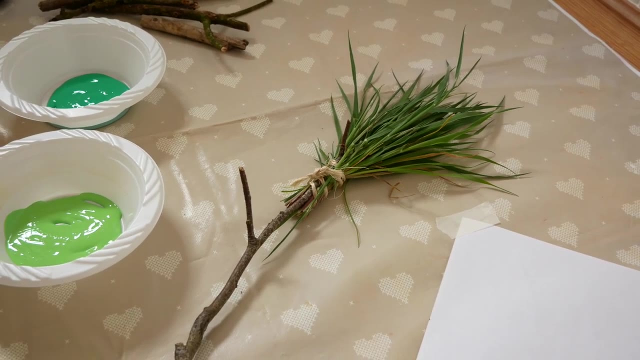 all things which i think will make pretty cool prints out for ben. i've also made this little paint brush using some grass, some twine and one of the twigs which i think should make some really interesting patterns. and then i've got some natural prints that i've put on my kitchen floor and i've taped some paper to the cloth using some 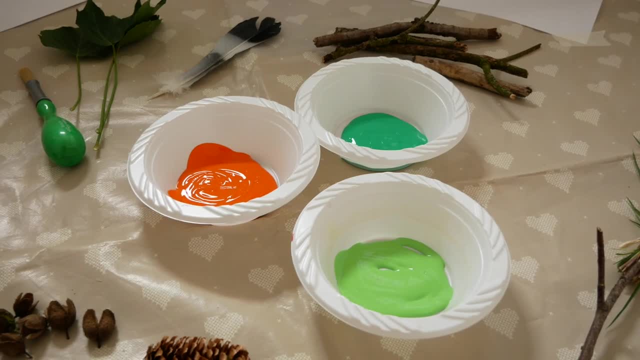 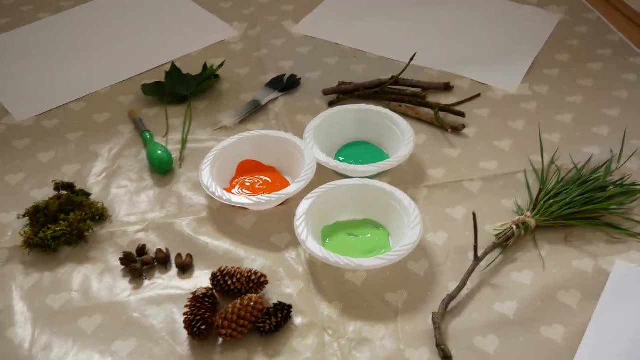 colored paints in the middle here. normally i put his paints in jars so that we can reuse them, but obviously a jar is going to be a little bit narrow for dipping pine cones and things like that into, so i've put it in some some bowls. but we will reuse these plastic bowls again for painting as well. 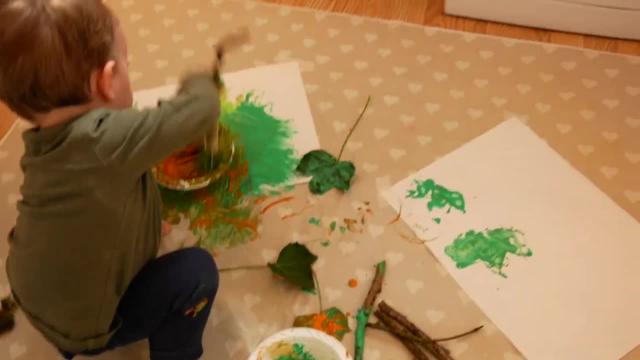 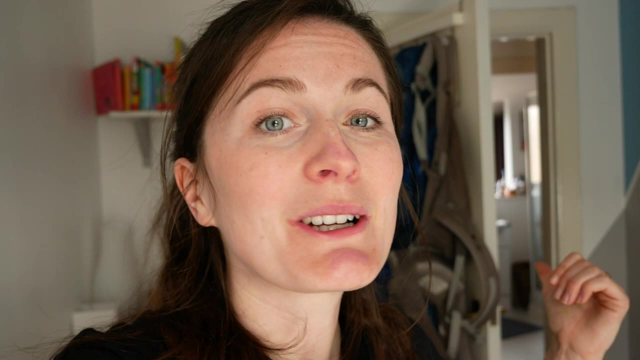 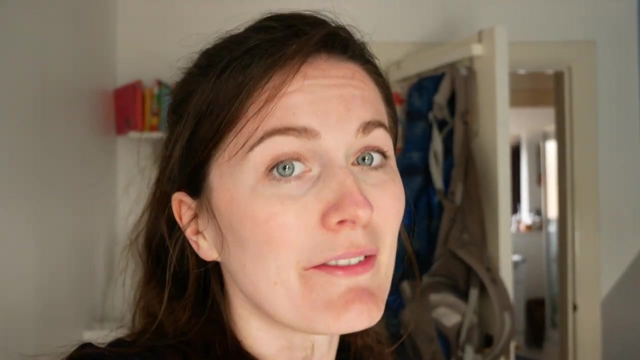 ben has gone straight in the bath because he was covered from head to toe in paint. you may be able to hear the shower going. he really loves having a bath, so this is another activity in itself. ben is really cranky this afternoon, so he didn't love that. 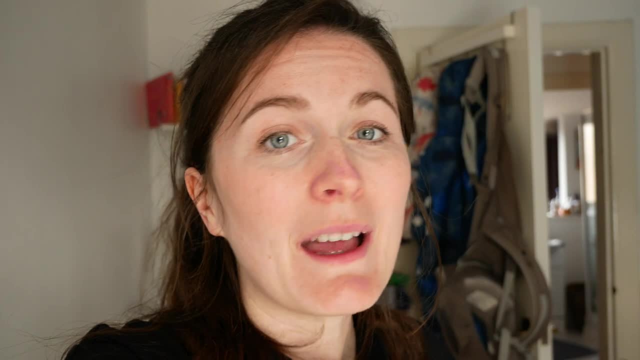 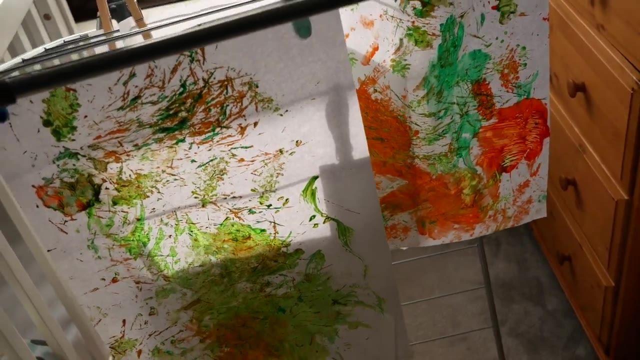 activity as much as i expected him to and as much as he normally would, but hey, that's toddlers. the finished pictures, though, do look really cool. this is one of kind of my arts and crafts hacks that i have mentioned before in other videos, so i'm going to show you some of the things that i've put in. 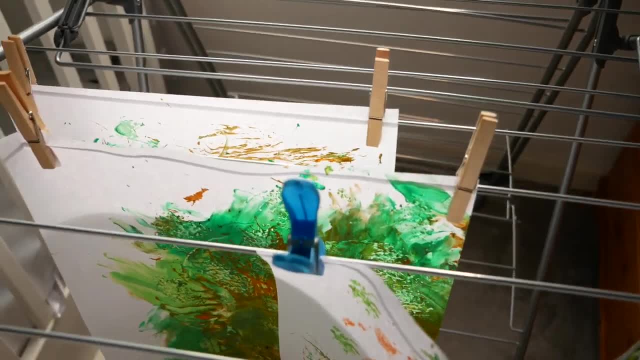 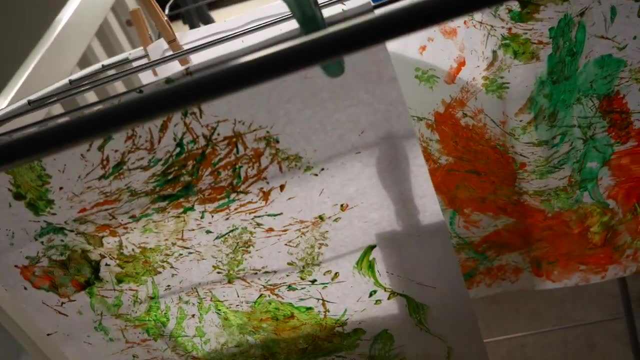 some of the videos, but putting them on a clothes horse means that they dry really nicely and stay out the way as well. i'm actually thinking about getting some frames, just just cheap frames, and putting some of this artwork inside for some family members. so those are my ideas for today. 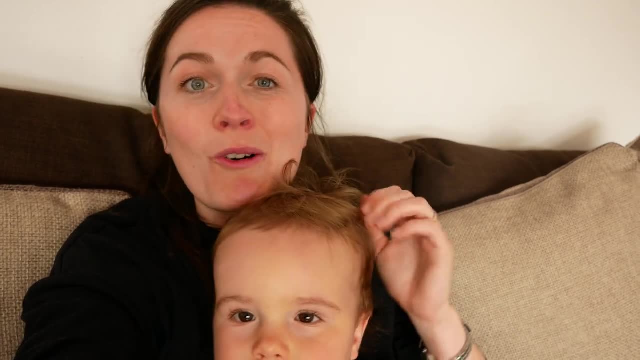 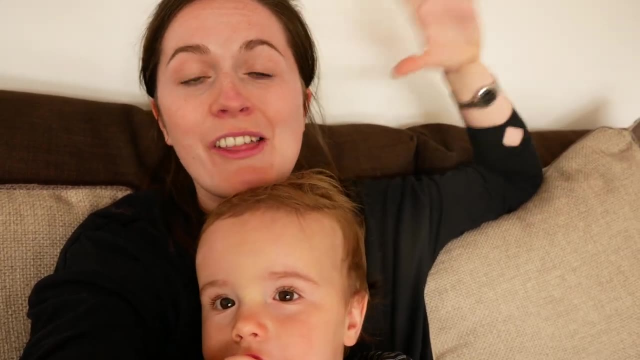 if you have other ideas- things that you do when you're out and about with your toddler, or crafts and and activities that you do with things that you collect- please let me know down in the comments. i would love some more inspiration and other ideas for things that we can do together. today has been 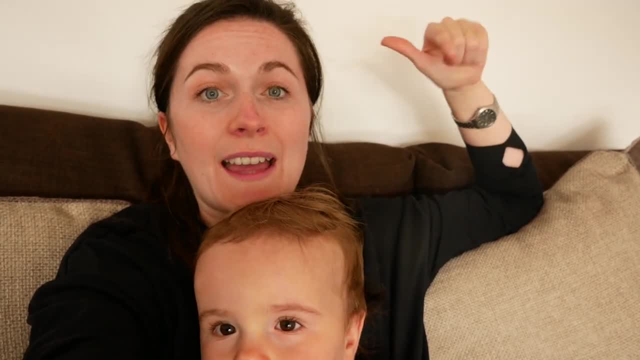 a bit of a pleasure to be here with you today. i'm going to show you some of the things that i've been doing with ben today and i'm going to show you a bit of a struggle for us, and i think that a part of that is to do with the fact that we have tried to do a lot of organized activities with ben.